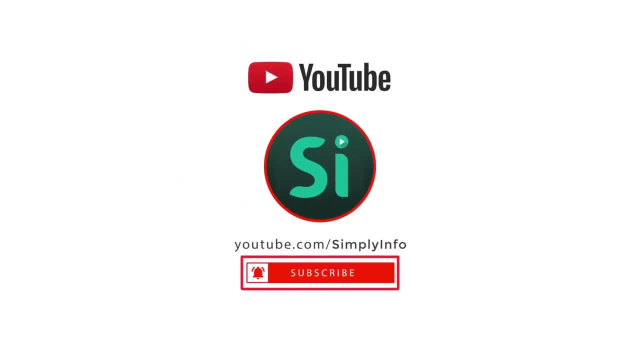 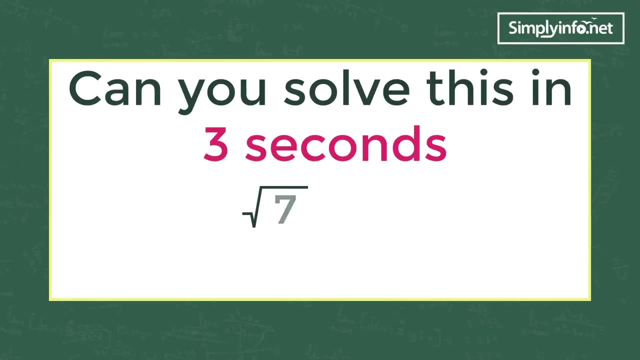 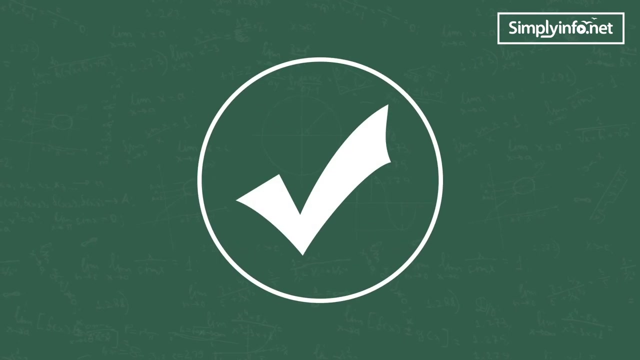 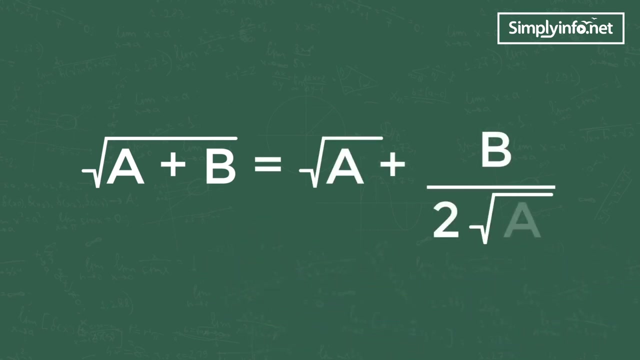 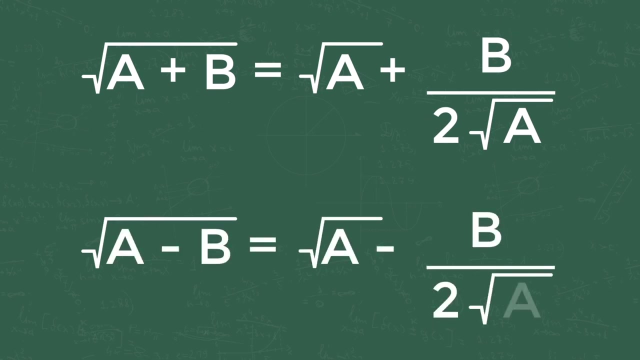 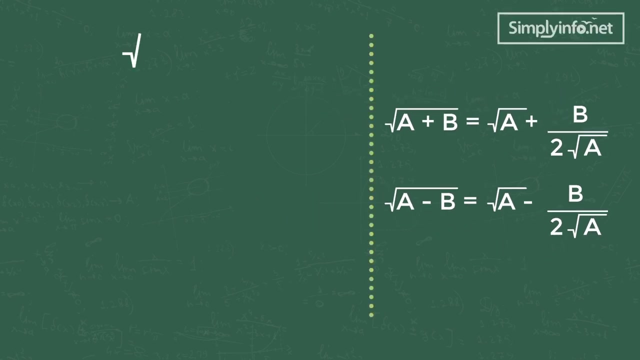 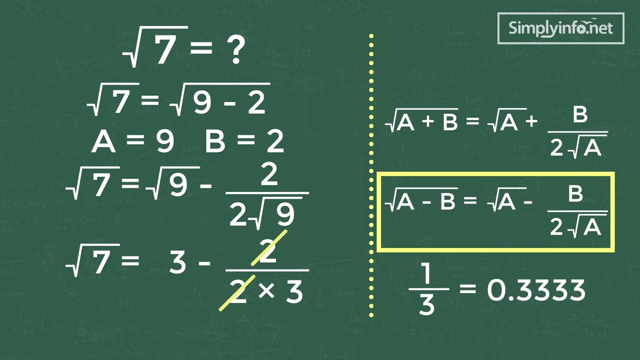 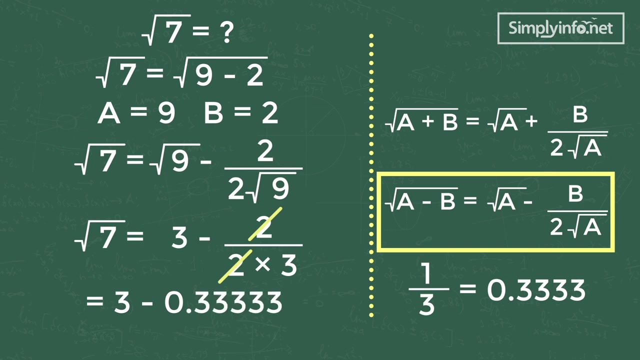 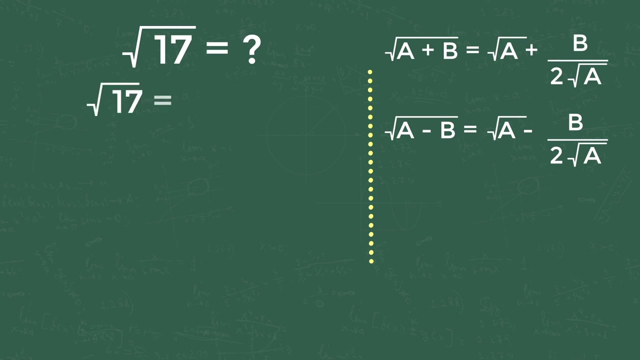 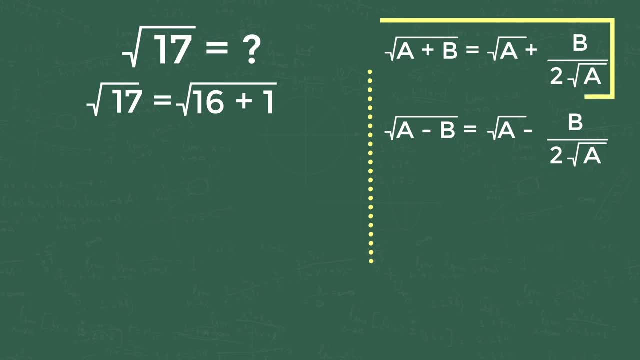 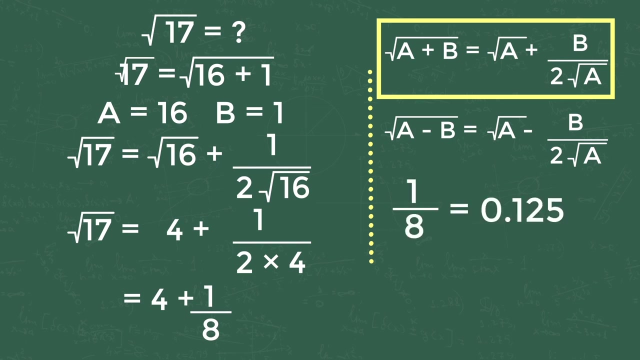 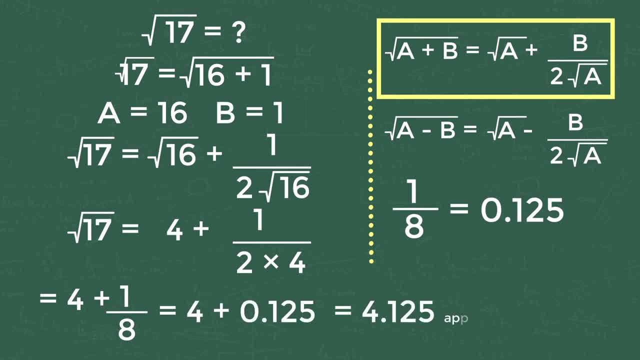 Please subscribe for more videos. Click the bell icon for updates. Please subscribe for more videos. Click the bell icon for updates. Please subscribe for more videos. Click the bell icon for updates. equals to 4.125. so the answer is approximately equal to 4.125. that's it. see how simple it is.